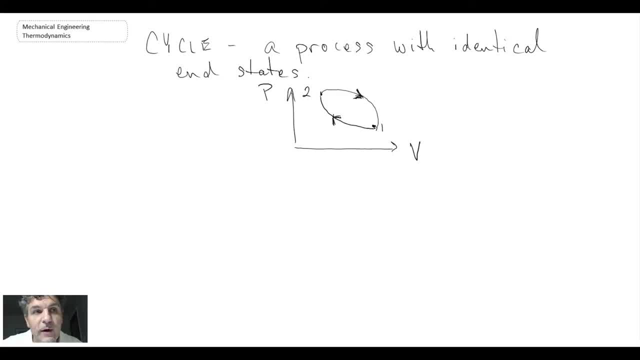 systems needed to be at equilibrium or within equilibrium in order to define the properties. Well, in reality, systems that we study are not in equilibrium, but what we do is we make a bit of an approximation through our modeling, And that is that we study what are referred. 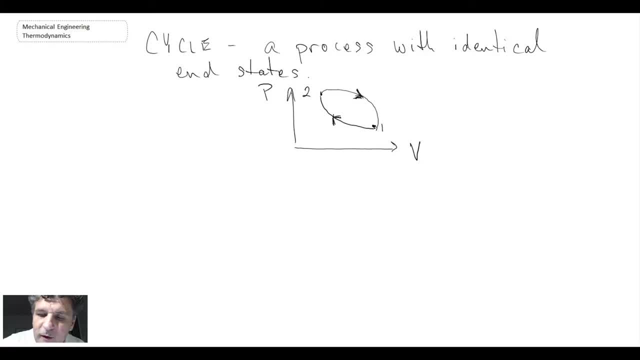 to as being quasi equilibrium processes. So let's define those quasi equilibrium processes And quasi equilibrium. what it does is it assumes that the system remains close to equilibrium. So it assumes that the system remains close to an equilibrium state during the process. Now, this is an idealization and really no cycle that we are really going to be analyzing. 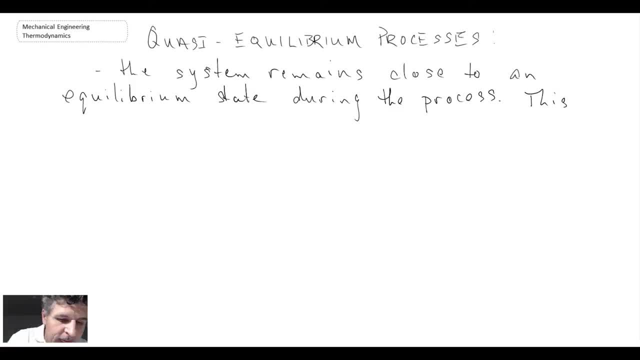 We will be in quasi equilibrium. So that is a pretty basic example of the process. But then we will talk about the free radical Yale model And what we found is that a very simple case. So if that's the case, why should we study them? If they don't really exist, why are we? 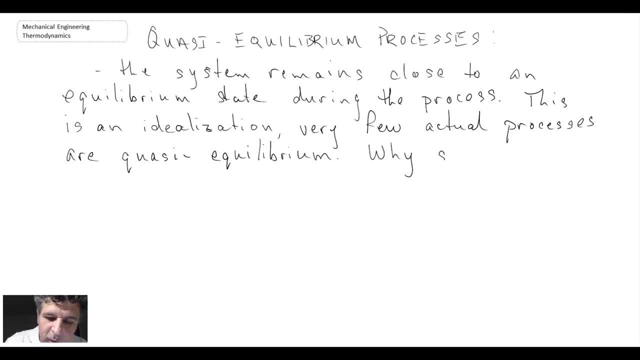 Well, there are a couple of reasons why we do study them. The first is that it makes our lives quite a bit simpler. They are easy to analyze. So that's the first main reason. The second is that work-producing devices, which is quite often what we'll be studying within thermodynamics-